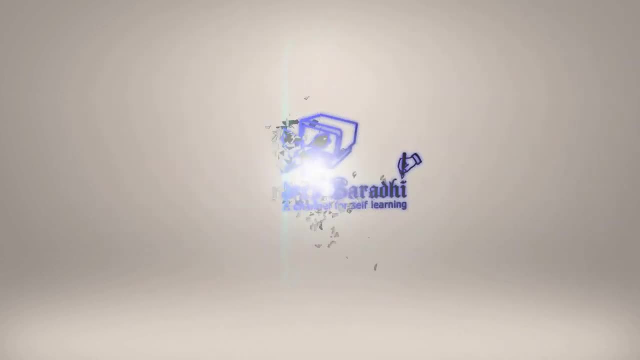 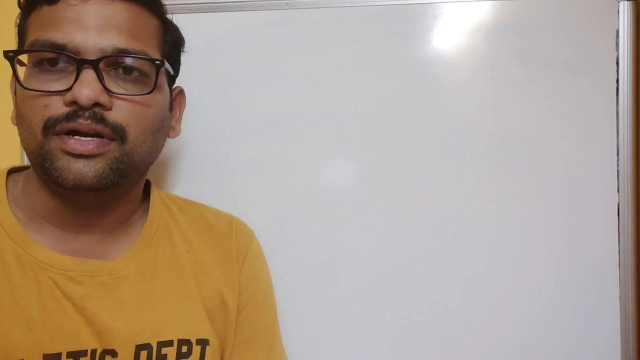 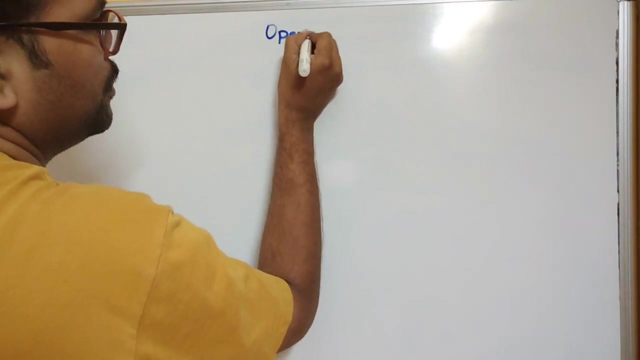 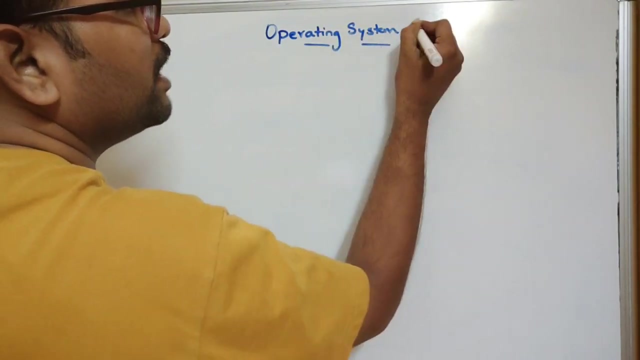 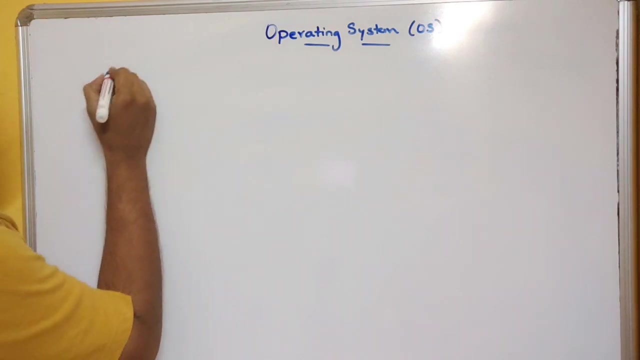 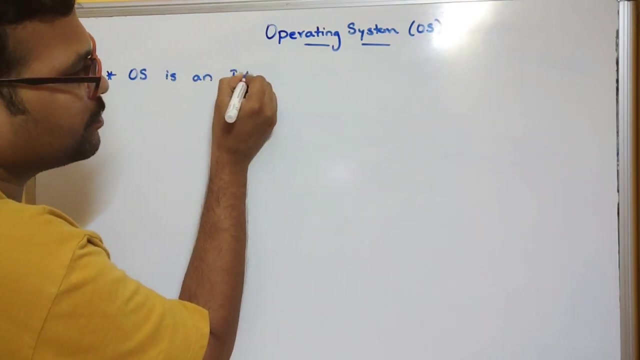 Hello friends, welcome back to our channel. So in today's session we will discuss about the introduction to operating systems. So usually this operating system we call as OS. So OS stands for operating system. So the definition of an operating system is OS is an interface. 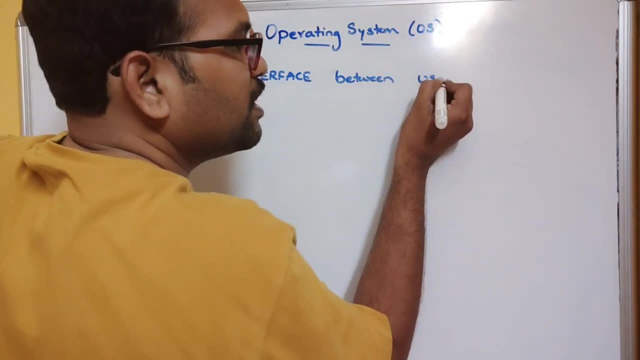 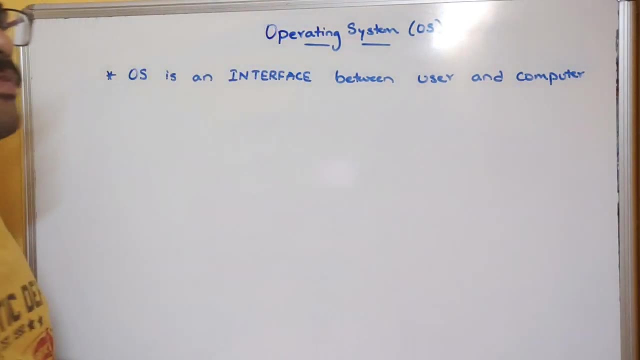 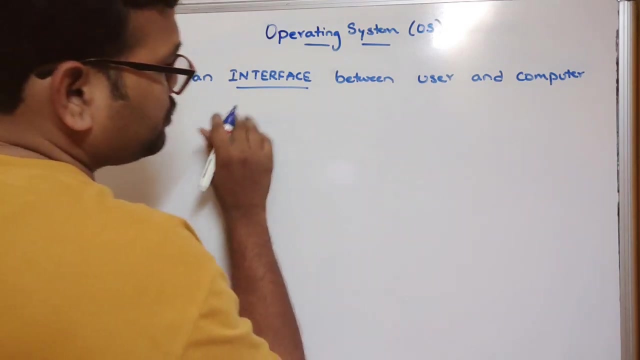 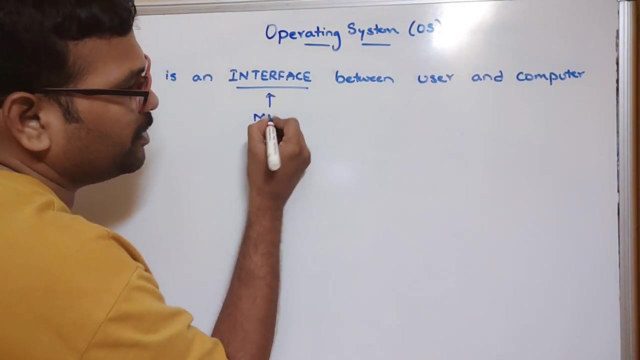 between user and computer. So I will explain about this individual word that is interface. So we are saying that operating system will act as an interface between the user and a computer. So what is this interface? This interface is also- I mean, for better understanding I am writing this one- So interface. 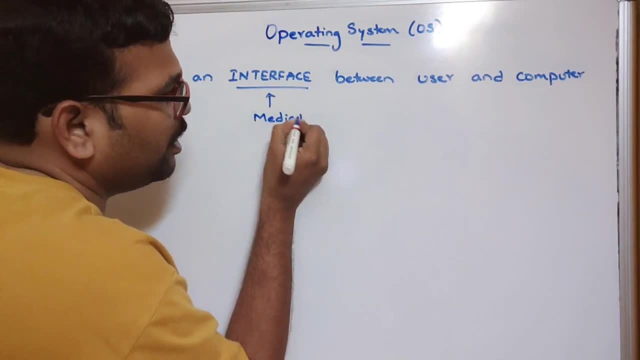 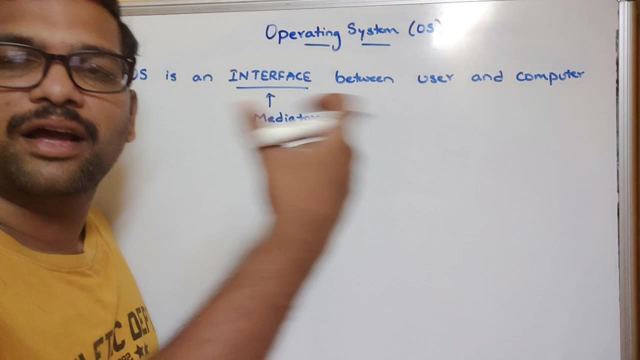 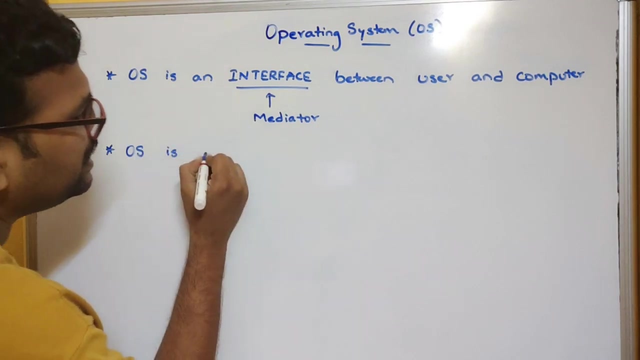 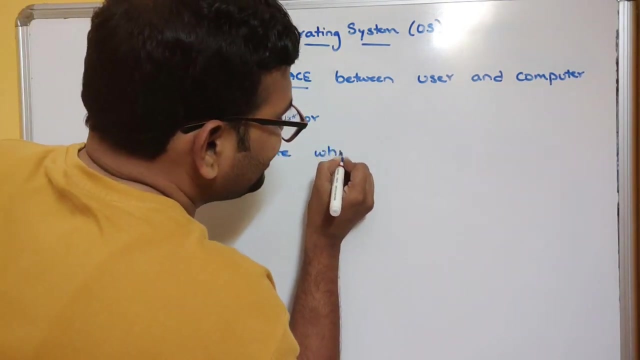 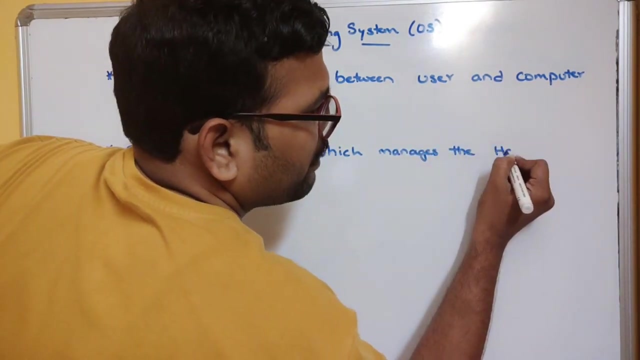 can be treated as a mediator. So mediator that means which is used for communication between the user and a computer. Okay so, and also the operating system is a software, is a software which manages the hardware, which manages the hardware right. So our computer will be having the hardware right. 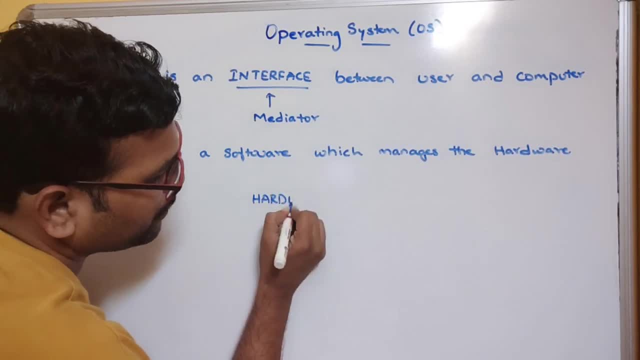 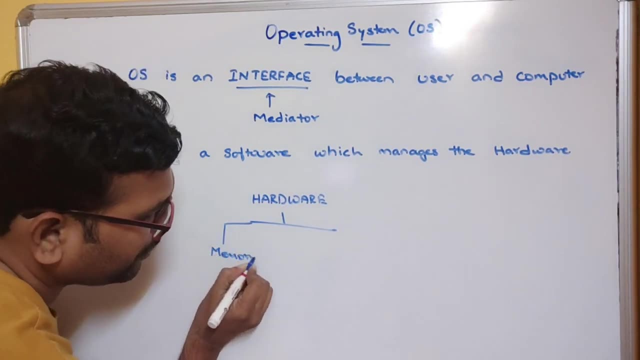 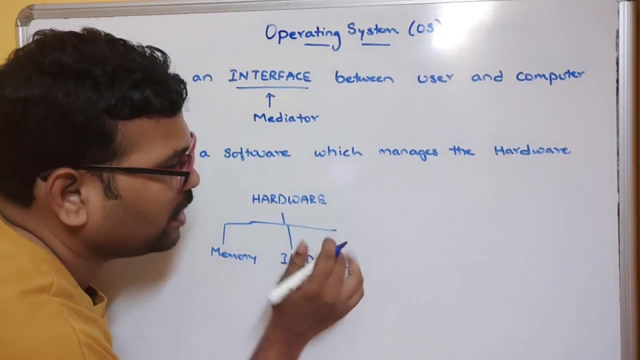 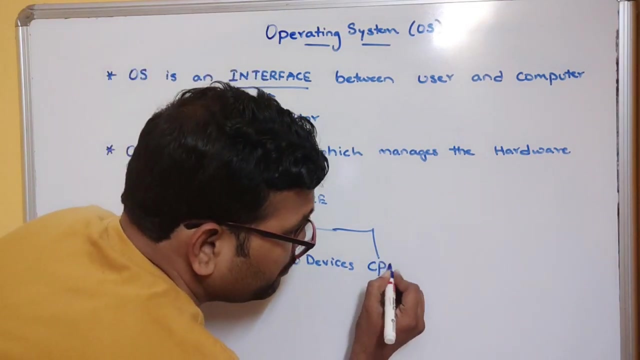 So hardware means so we will get the memory, I O devices, etc. everything will be comes under this hardware right. So CPU, main thing. we have forgotten about this main thing. CPU that means the processor and etc. So everything we call it as an hardware right. 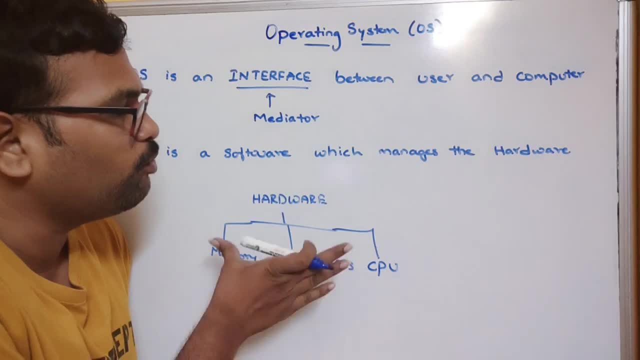 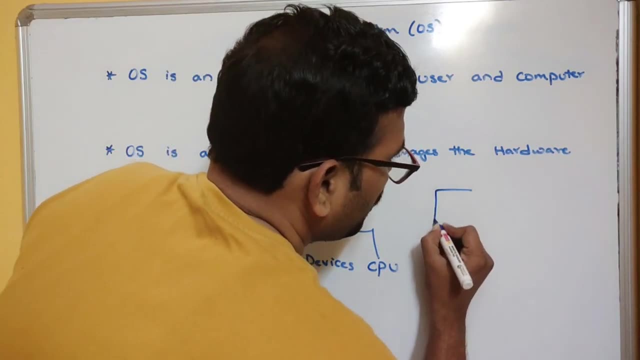 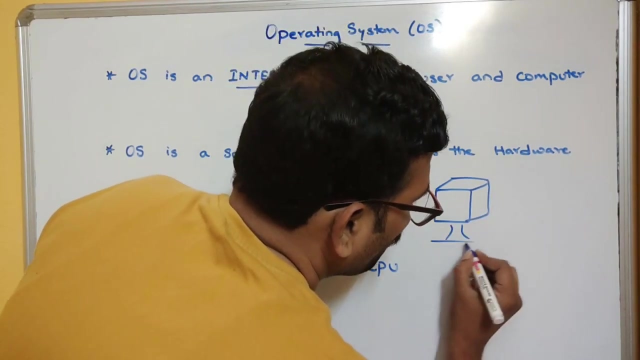 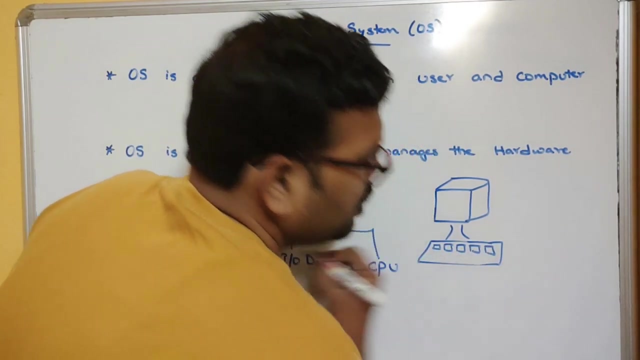 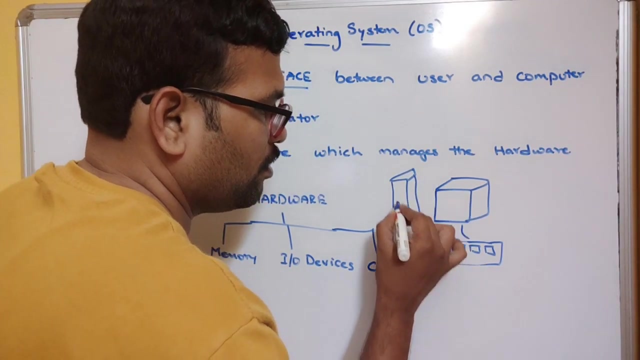 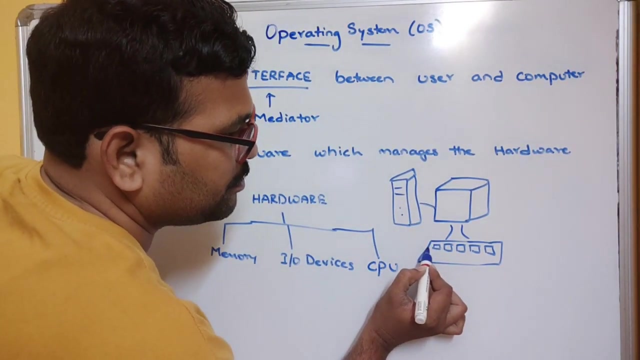 So, in order to communicate with all these things, we require one software which is called this operating system. Best example: so consider a computer. So here we are having some sort of keys. So we are having some Okay Keys, right, So there will be some okay. 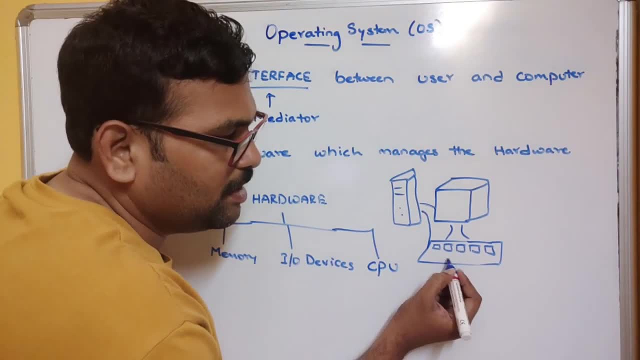 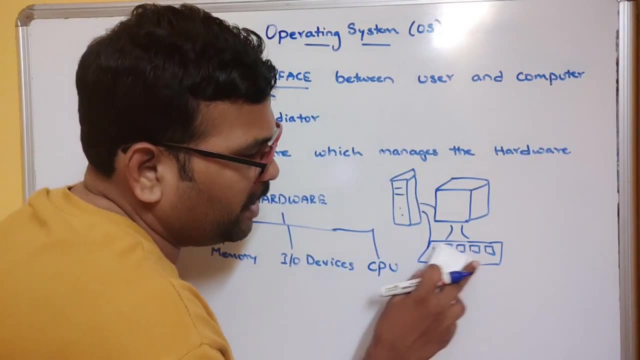 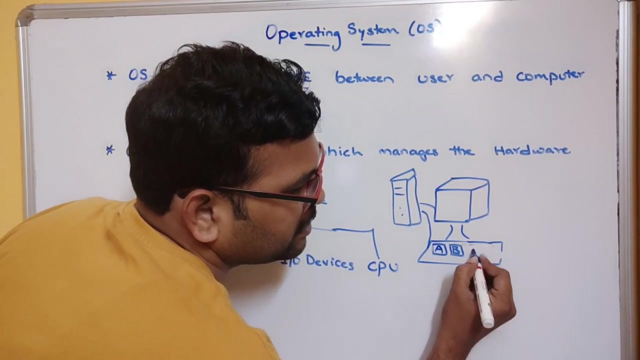 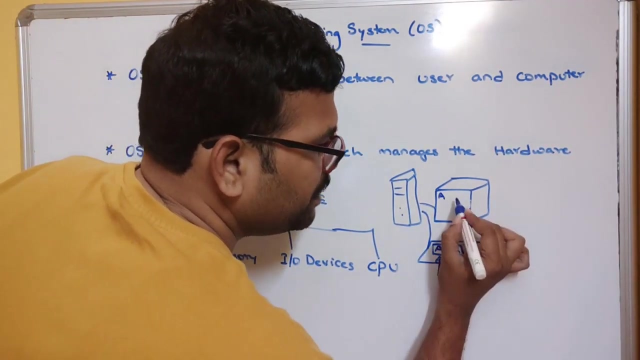 So if you press these keys- okay, if you press these keys, the key will be printed on the screen. if you press A, for example, we will be having all the keys here. So, for understanding, I am writing only A, B and C. okay, So if you press A, the A will be displayed here and immediately. if you press B, B will. 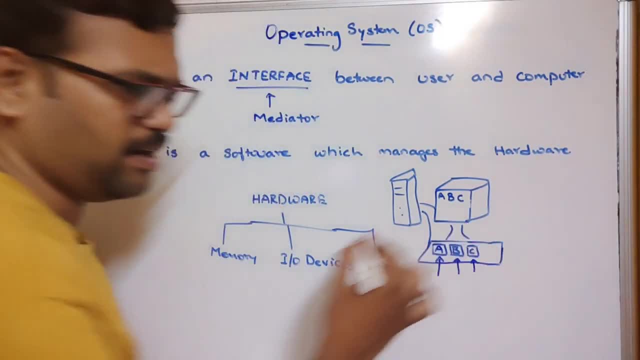 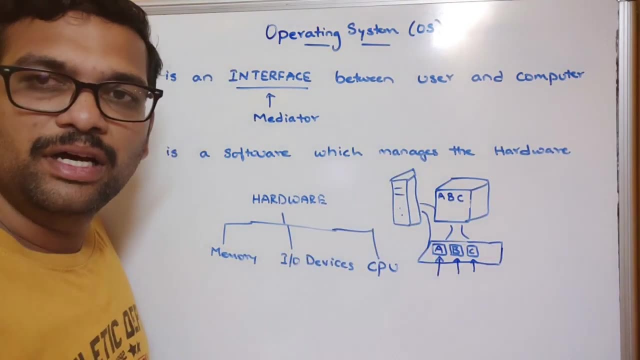 be displayed, and if you press C, the C will be displayed here and etc. right? So whatever the input we are giving from the keyboard, immediately the same thing will be appeared on the monitor itself. right? So this happens with the help of a software called. 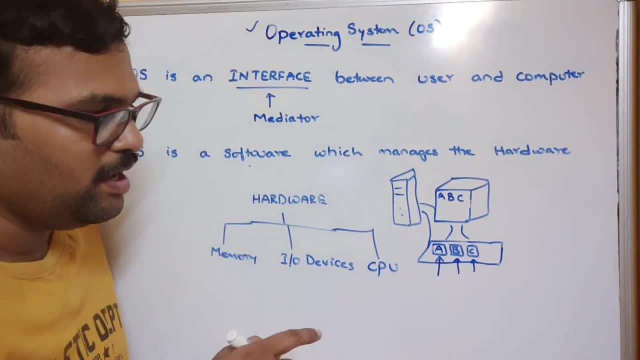 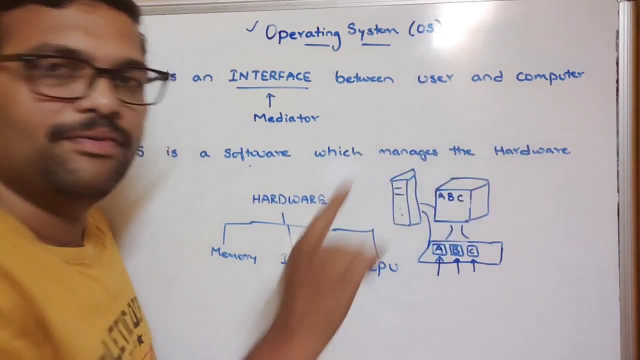 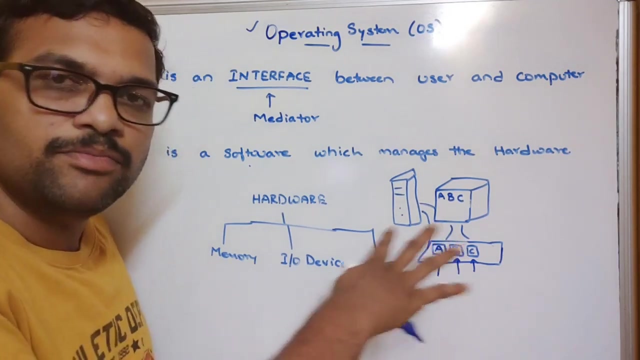 So this happens. This is called operating system. So that's why that's why we are saying the operating system is a software which manages the hardware right. So here we are interacting with the computer, right, We are interacting with the system with the help of some sort of hardware, right? 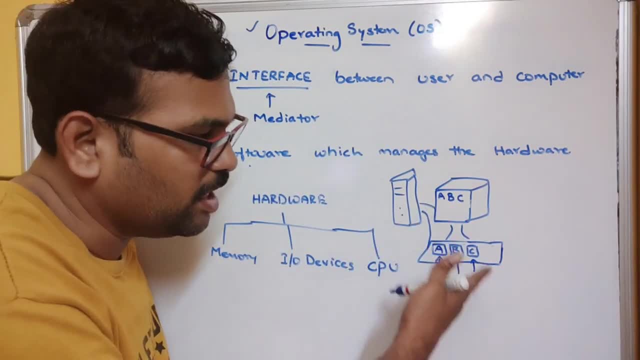 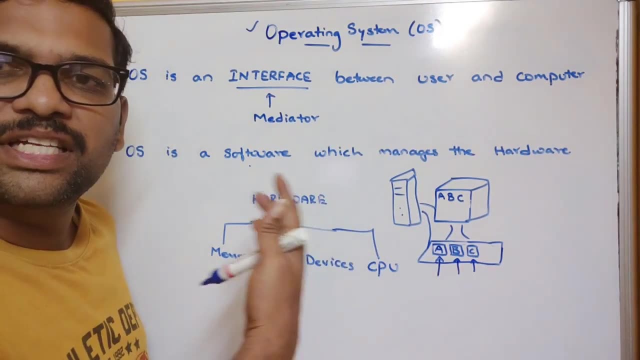 So here we are using some input devices, So input device like a keyboard or a mouse right, and we are getting the output in the output device. So there must be one interface between these things. So what we are giving the instructions and what the system understands, everything will. 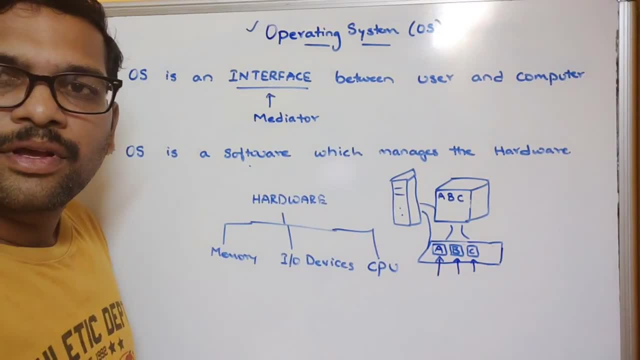 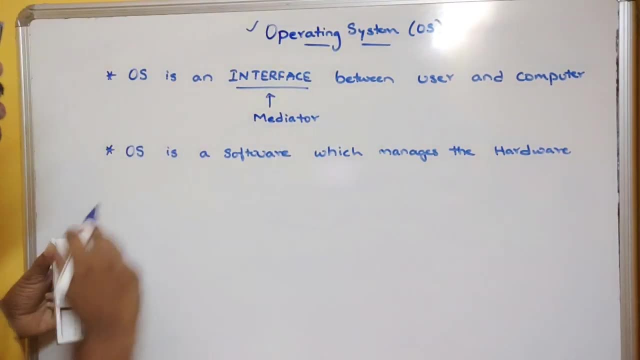 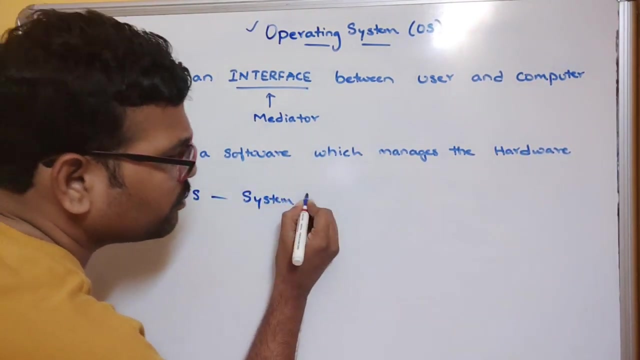 be done with the help of this operating system, right? So let me give you a diagram for this one for better understanding. and also, the operating system is a system software. It's a system software. So we have seen in the previous sessions about the categories of softwares. that is a system. 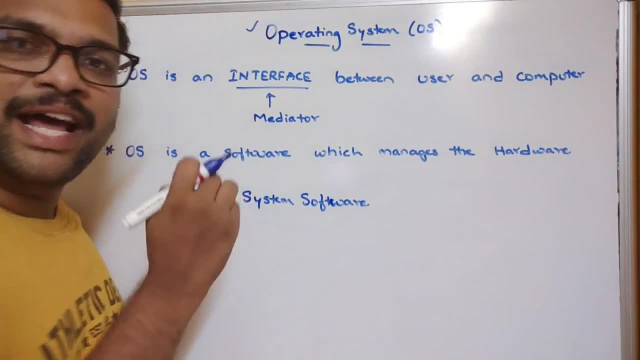 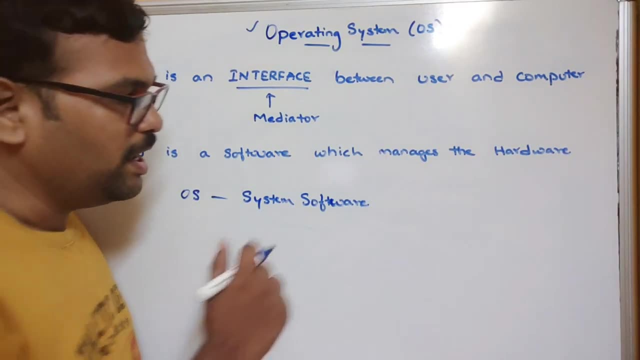 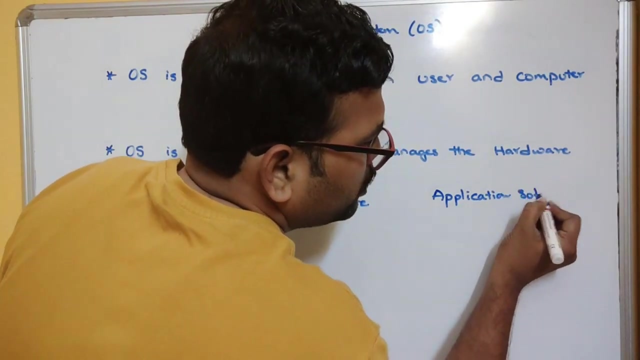 software and application software. So system software means which manages the hardware, is called the system software. Okay, The software which manages the hardware is called the system software and another one is an application software, application software, So which we call it as an application software. 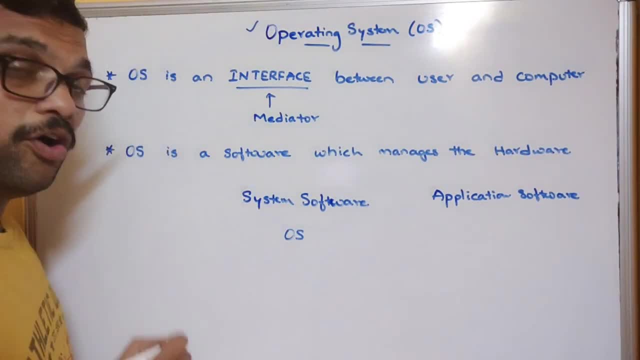 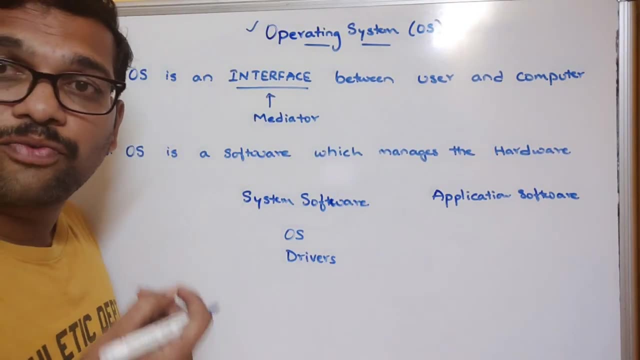 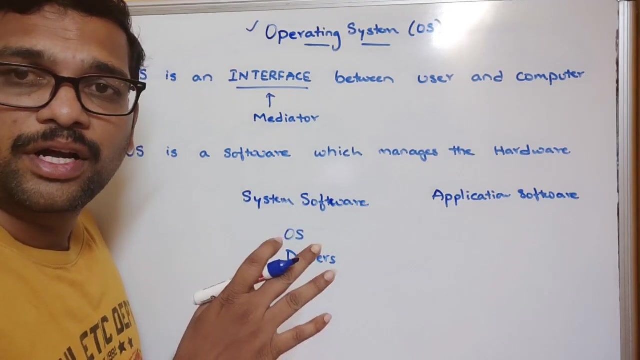 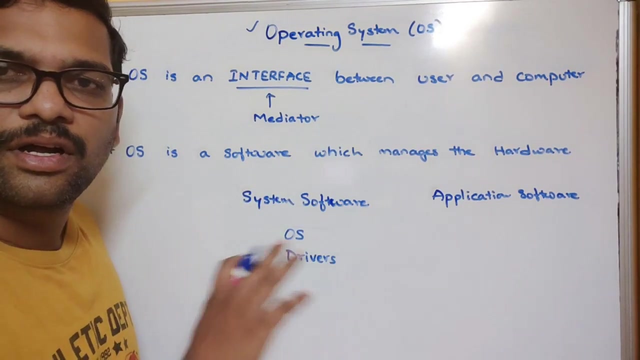 So here the example is operating system and also some sort of drivers, drivers, software drivers. For every hardware there will be a some sort of software. So unless you install the software the hardware will not be get work right. So some operating system will get these drivers inbuilt. okay, with the operating system, that's. 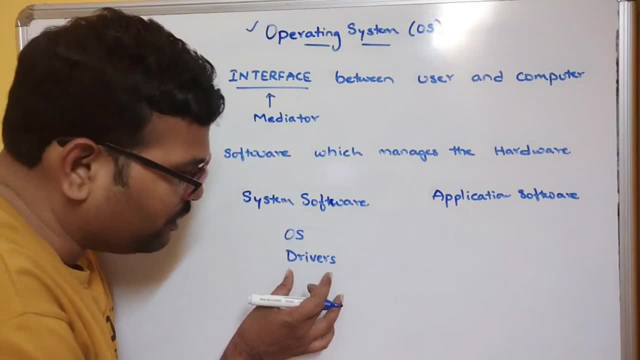 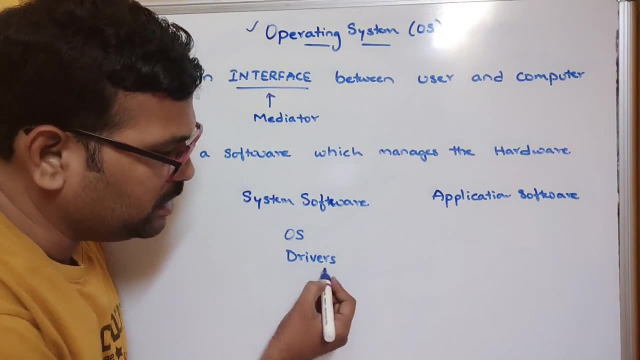 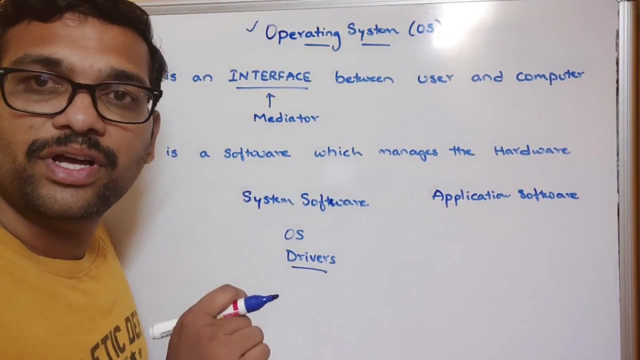 different right. So every hardware will be having the drivers and to work the hardware properly we have to install the drivers, and these drivers are also known as the system software, And application software is a system software, So application software, these are the softwares which are meant for a specific task or functionality. 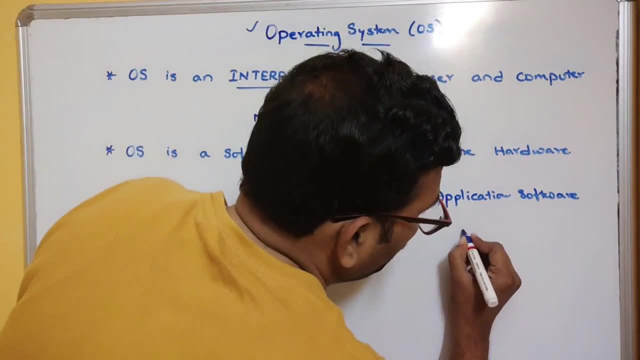 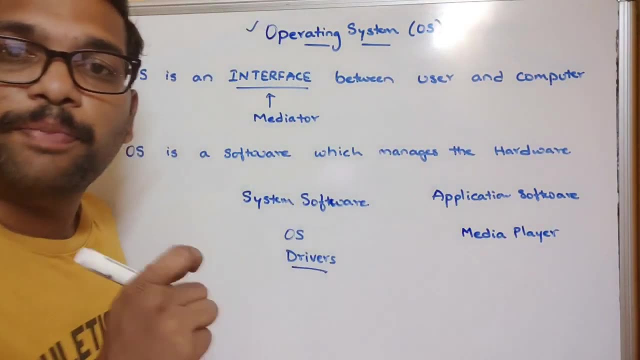 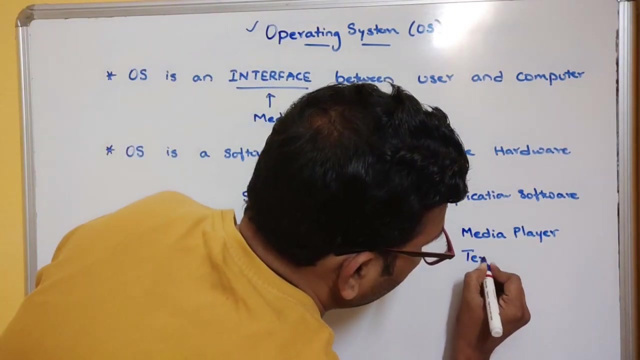 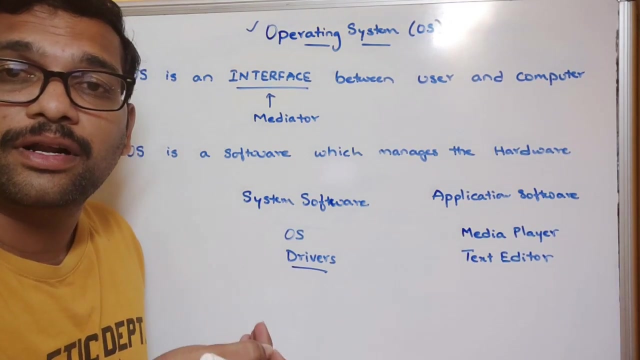 some specific application, for example, some media player, So this software is used to play the media. that means either audio or a video, okay. And text editor, text editor. So this is a software which is used to play the media. Okay, This software is used for writing the text, okay. 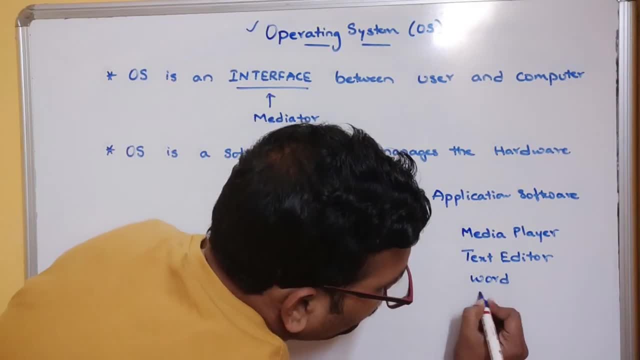 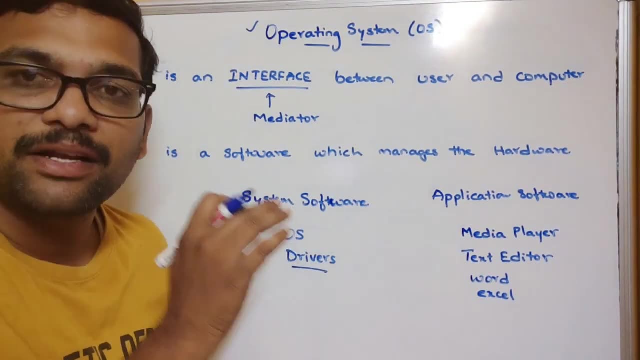 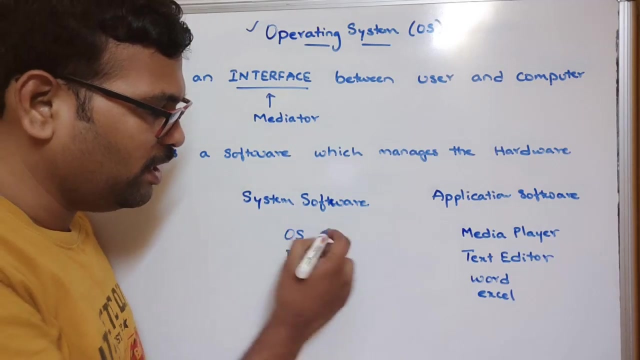 So like word excel. so all these are nothing but application software. application software, So these are meant for a particular task. okay, System software, which manages the software, I mean which manages the hardware, is called the system software. We are having two types, that is, the operating systems and the drivers. 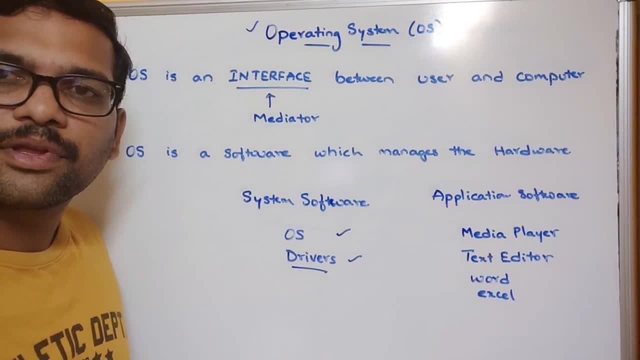 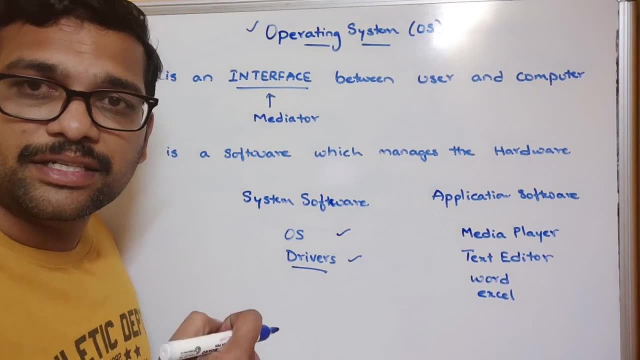 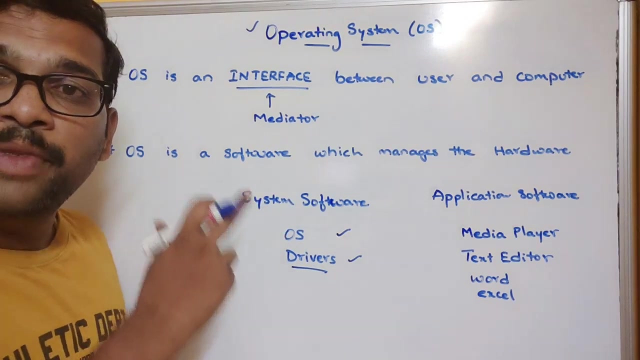 So without operating systems we can't interact with the system. okay, So we can interact, but we have to pass each and every instruction, each and every instruction. So it would be very difficult for the user to interact with the computer without operating system. So, to make the user easily accessible, this operating system will help, okay. 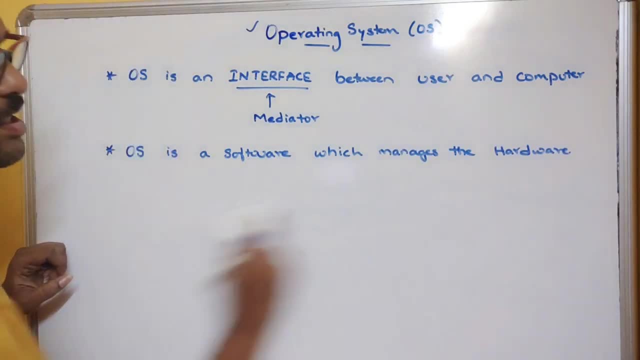 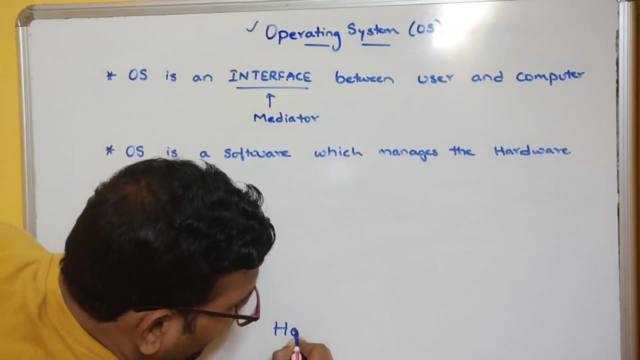 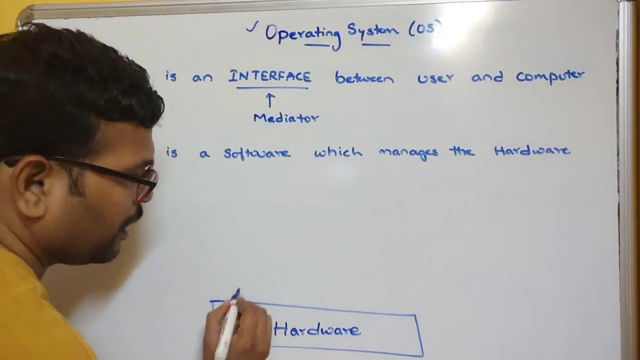 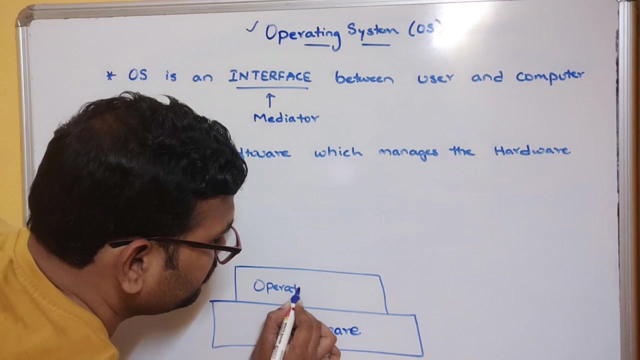 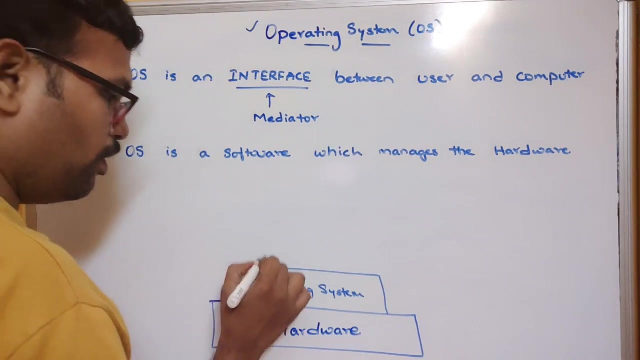 Now let us have the structure of this operating system, So the importance, importance of operating system, So the lower, So the lower. Okay, So this is hardware, so this is the hardware, and here we are having the operating system because this operating system will manage, as the hardware right, and this operating system. 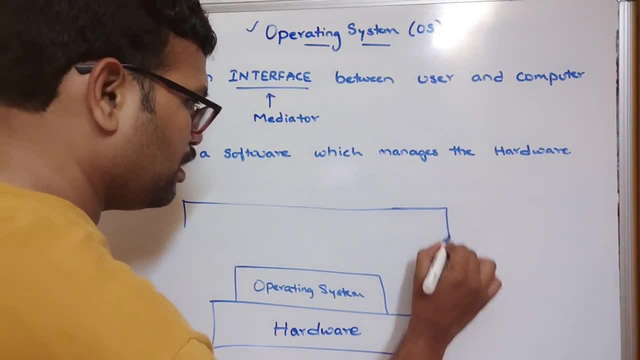 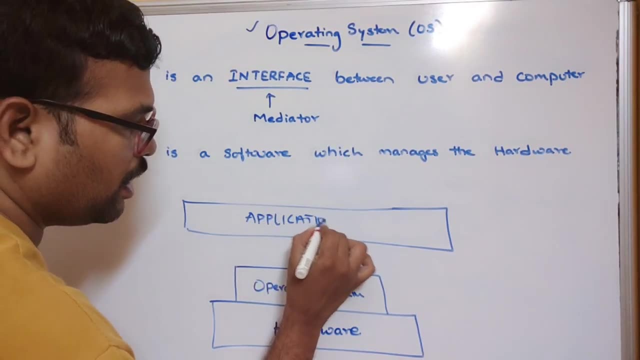 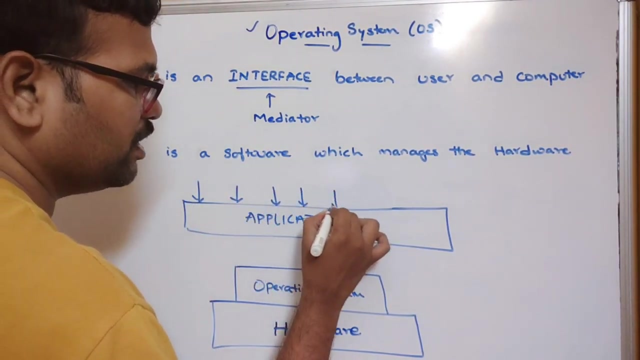 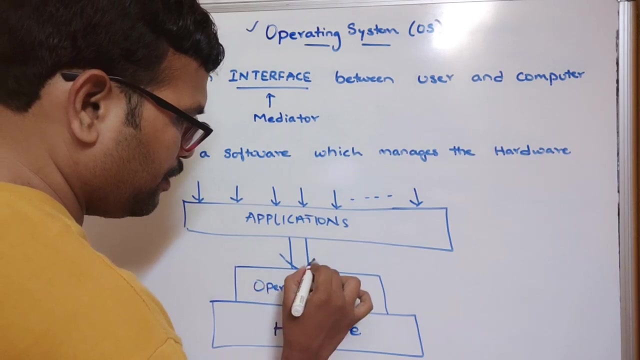 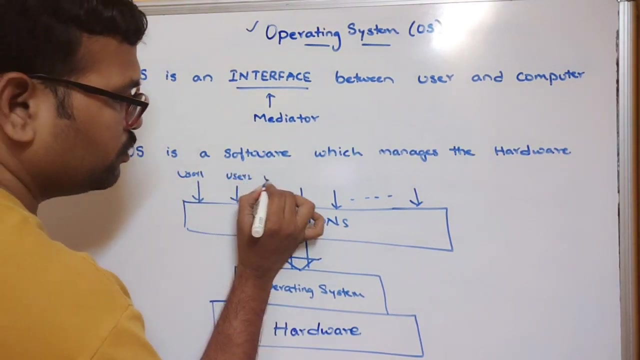 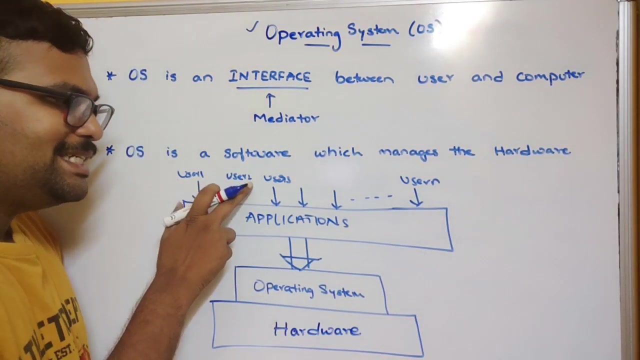 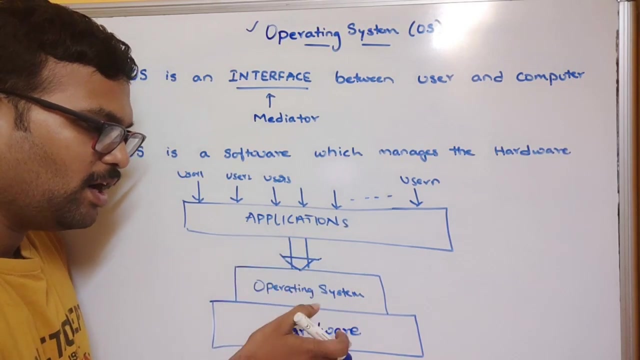 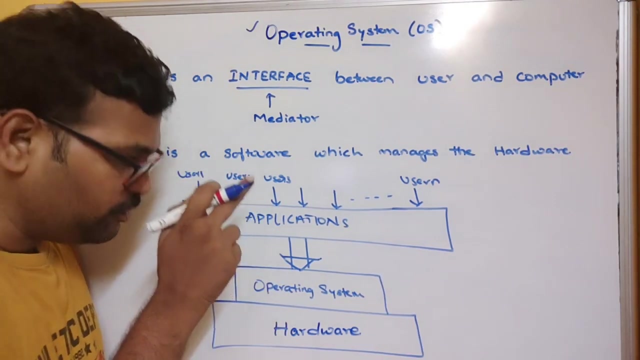 again we are having Okay, Okay, And here we have the three applications. Okay, and here we will be having the users. here we will be having the users, right, So user one, user two, user three, and so on. User n, So number of users, can be applied. So these users will use the applications and these applications will be implemented or executed by the hardware with the help of operating system. Okay, So these are the applications and in order to run the applications, we require the operating system. 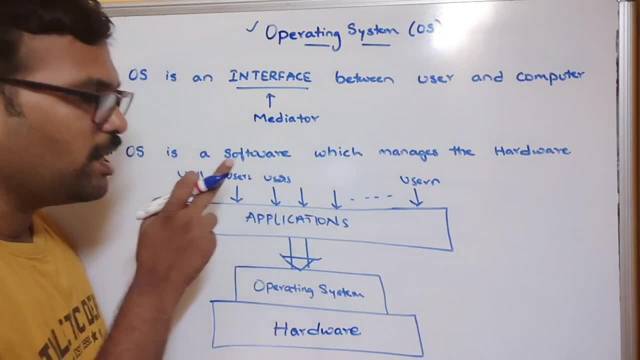 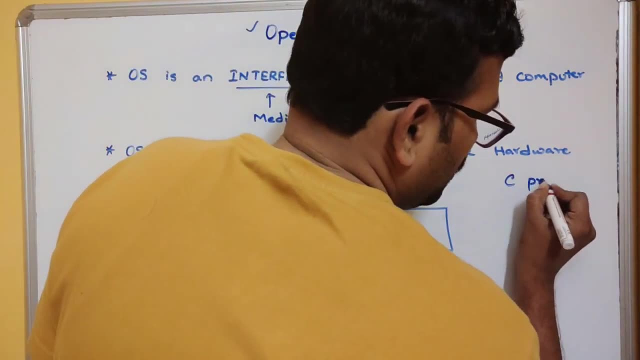 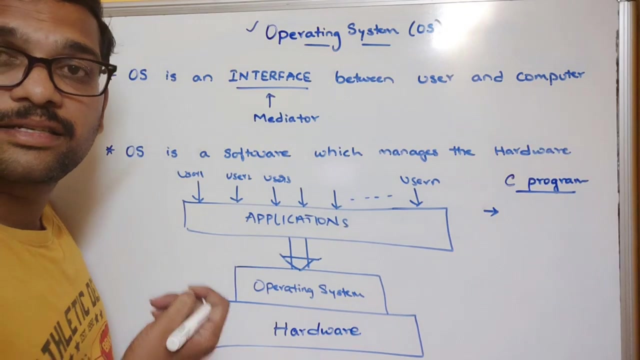 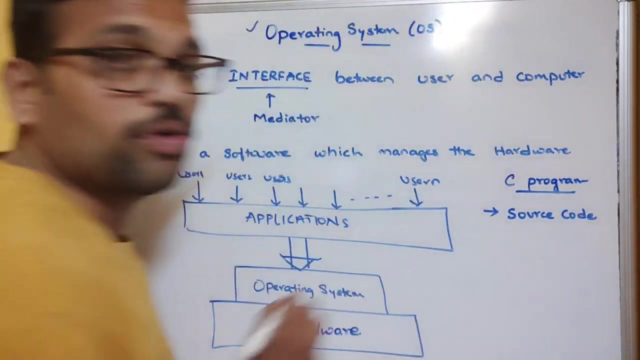 Okay, So without the operating system we cannot run these applications. Example: let us take the C program. Let us take the C program. So the first step, we will write the instructions, We will write the instructions and we will save the file with the c. So that is a source code. So we will prepare the source code for a C program. 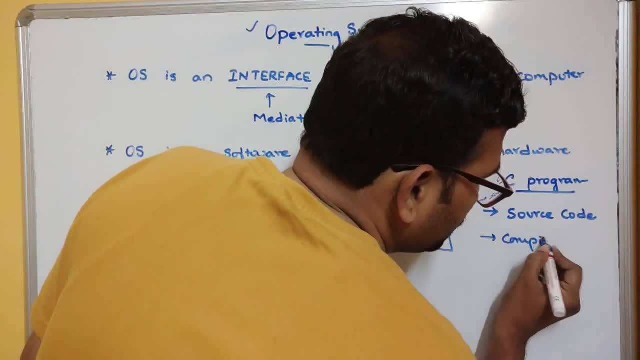 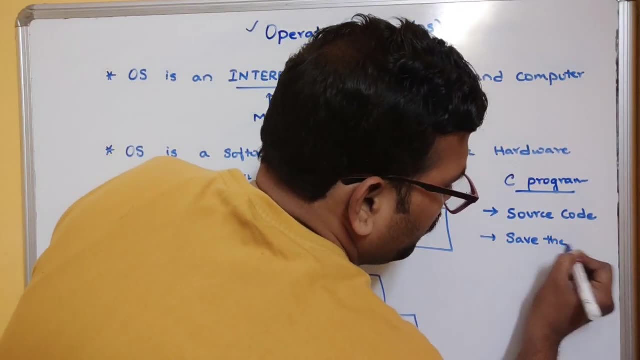 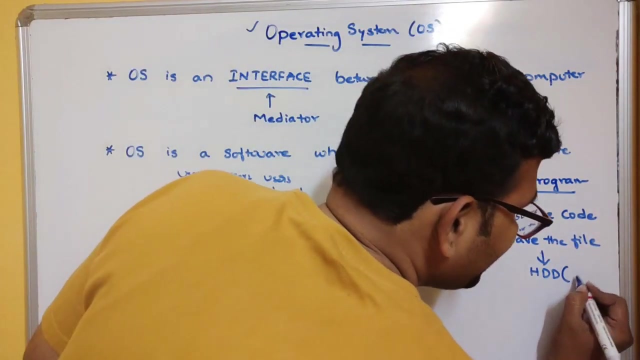 And the second step: we will do the compilation process. So we will save the file. Okay, We will save the file. Save the file, Okay. And where it will be stored? It will be stored in hard disk. Hard disk, That means secondary memory. 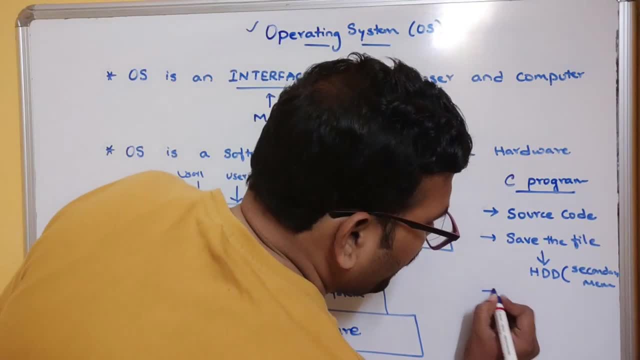 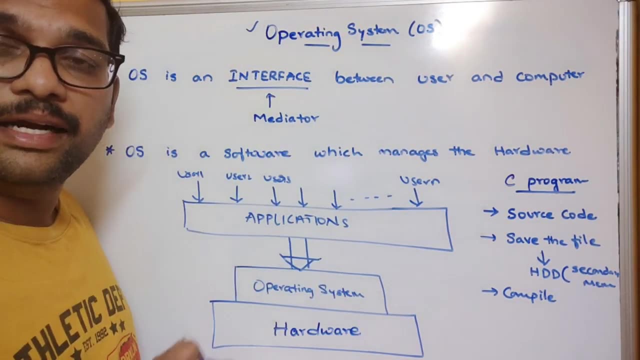 Secondary memory. So hard disk means secondary memory, And again after that we will use the compilation process, Compile the program. Again, that will be in hard disk itself. Okay, Okay, Okay, Okay, Okay, Okay, Okay. 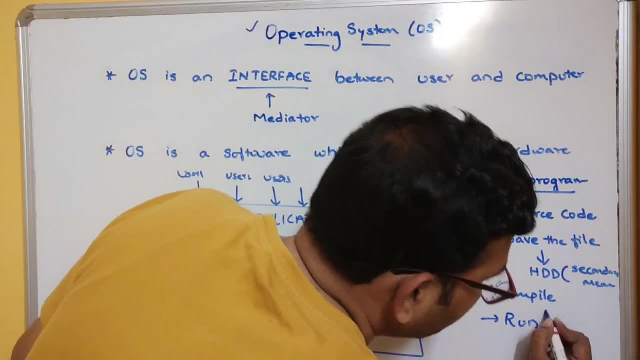 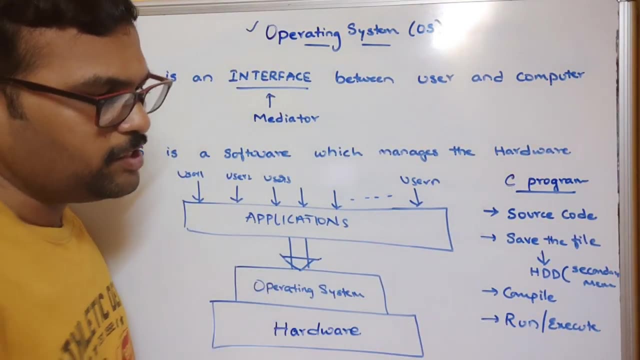 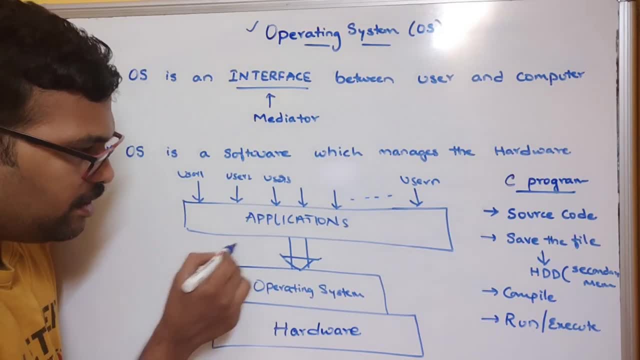 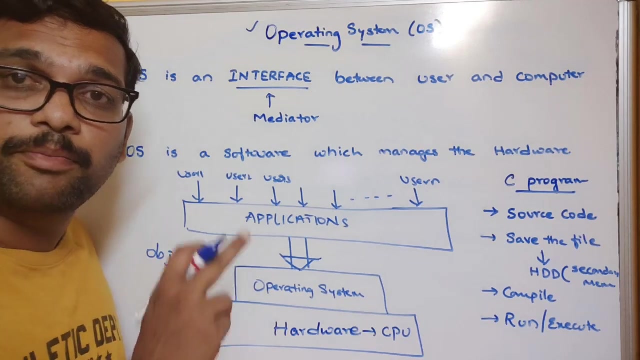 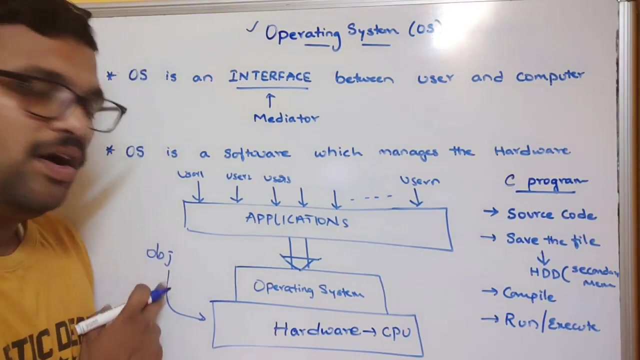 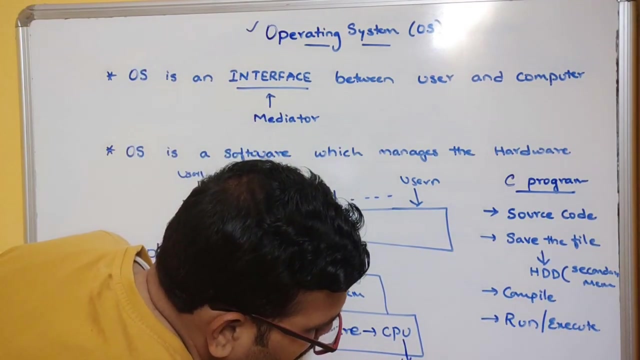 So the object file will be given to this particular hardware Right. The object file generated by the compilation process will be given to the hardware Hardware. here is nothing but CPU, So all the applications will be given to the hardware. Applications will be executed by the processor itself. So our system is having some processor, So that processor will execute the object code and this CPU will access only the main memory. 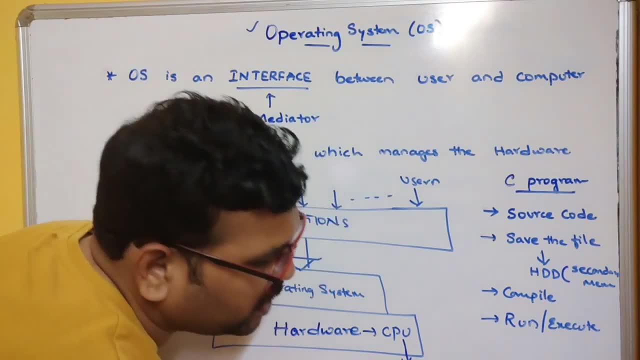 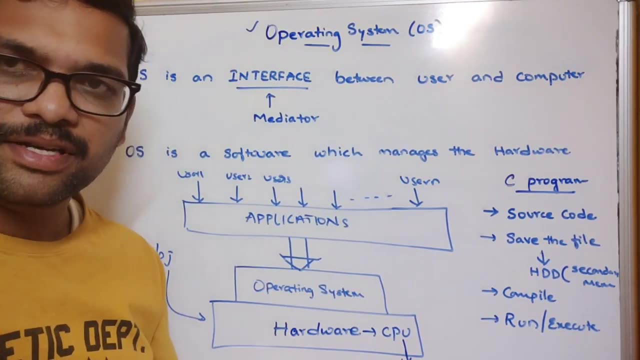 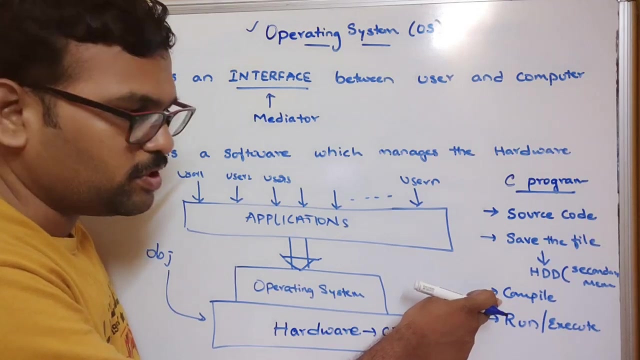 The main memory, So it will not execute the applications from the hard disk. It will execute the applications or processes from the main memory itself. So during the running or execution, the object file generated from the compilation process will be stored into the main memory and it will be available for executing by the processor. 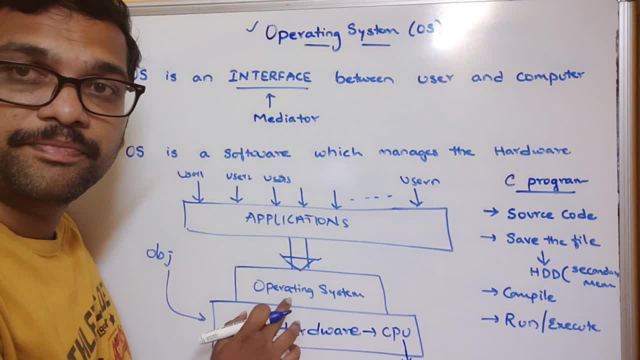 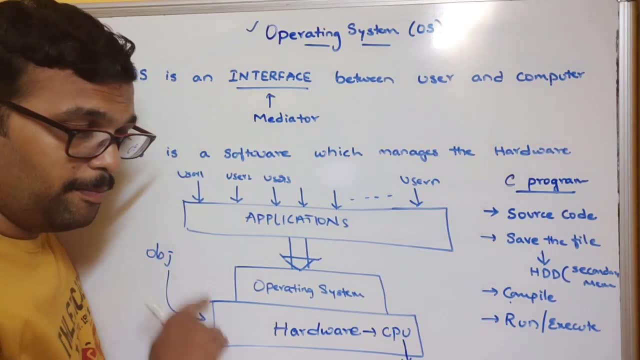 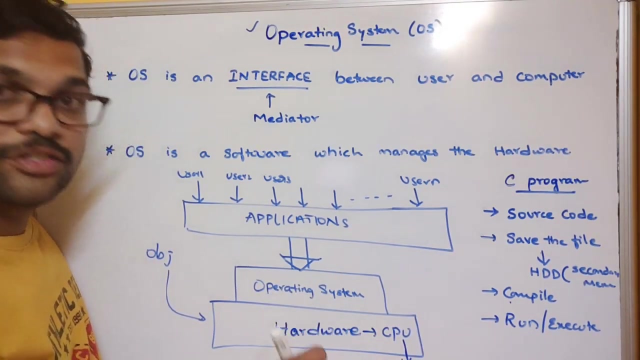 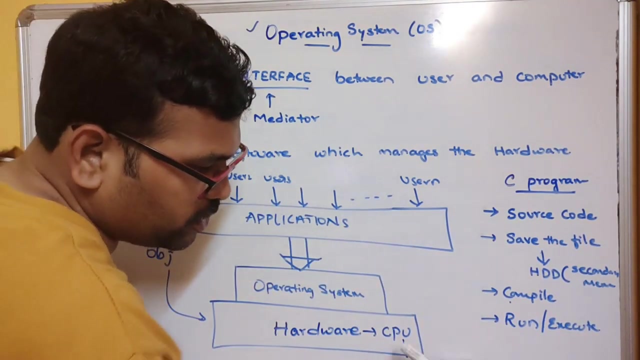 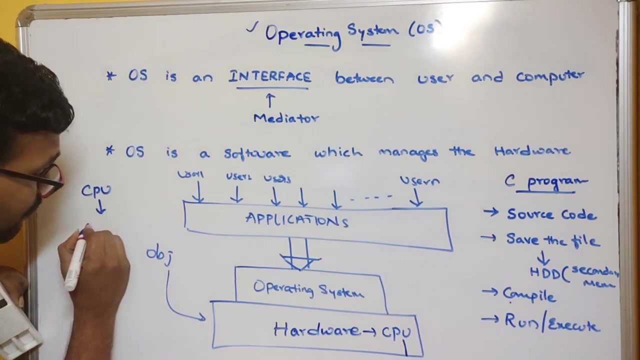 And all this process will be done by the operating system. So hope you understood. So, once the compilation process is done, we get the object file and see, remember, every process will be executed by the processor itself, Every process. So here. so we are saying that execution of a program is also a process. right, Execution of program is also a process. and see, the CPU. CPU will access everything from the main memory. 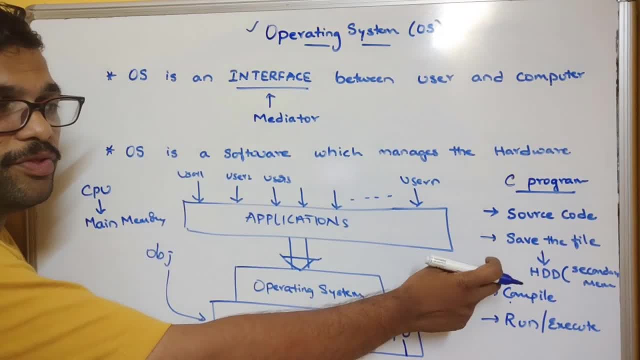 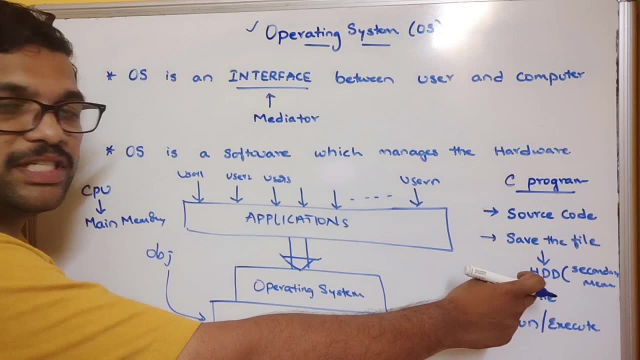 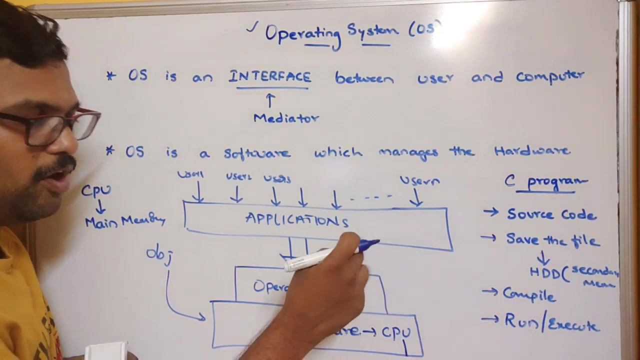 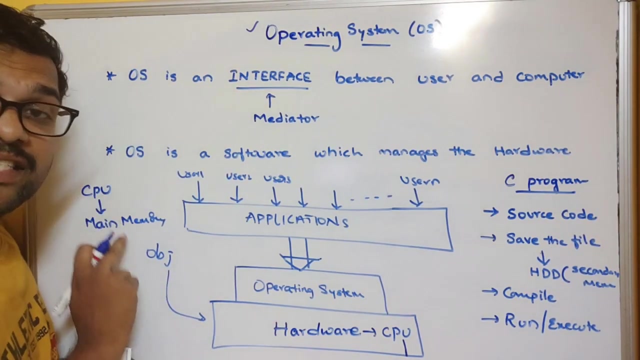 But the files are in secondary memory. So now during the execution the object file which is generated from the compilation will be stored into the main memory. That means it will locate or it will load the object file to the main memory, because the CPU will execute the processes from only the main memory. So this process will be done by the operating system. 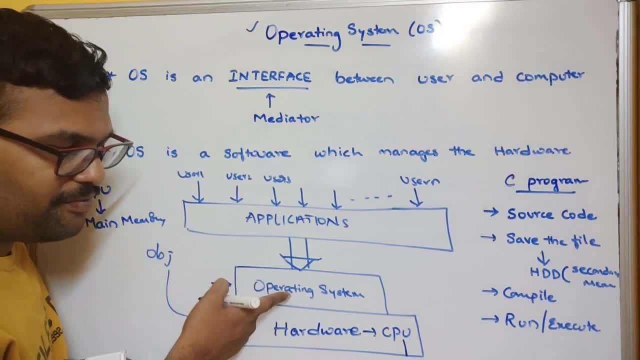 So that's why operating system is an interface between the user and the hardware. If you want to execute any programs, so that programs will be done in the applications and that will be executed by the CPU with respect to the operating system, with the help of operating system right.